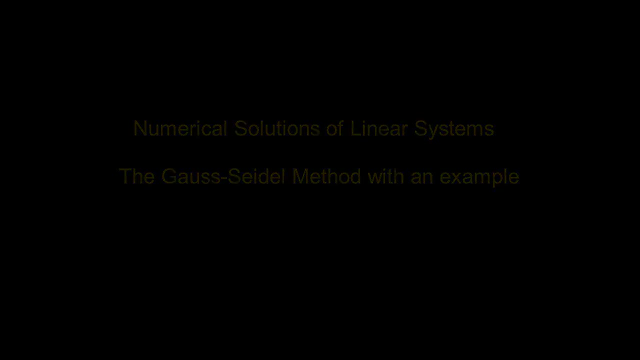 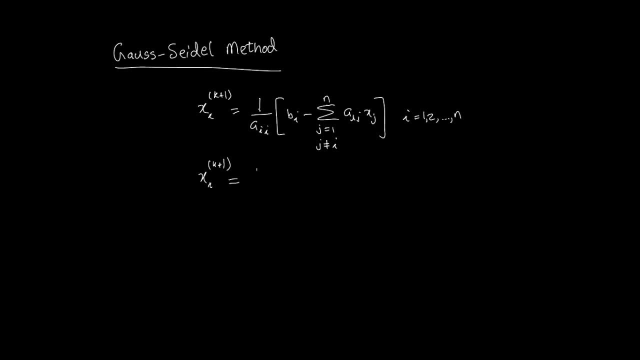 xi k plus 1 equals 1 over, and let's go with the first equation. for instance, If I go with, for instance, x1 for the sake of argument, then this becomes a11 times b1 minus. now let's start looking at this. So we're going to get 1, 1, x1, okay, and then so I'm going to leave this: yeah, minus a1,. 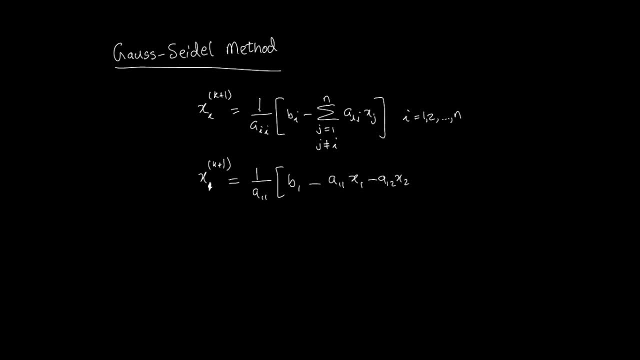 2,, x2,, okay, and so on. okay, So that's the first equation that I'm going to get. So this is going to go up to 1n, for instance xn, and that I'll stop there. Now, that's for i equals 1,, of course, that's the first equation. In a similar way, I can get the second equation. I want you to notice something. Sorry, I forgot those k's which I've just introduced back there now. so k at the root. Now see those k's. so okay. 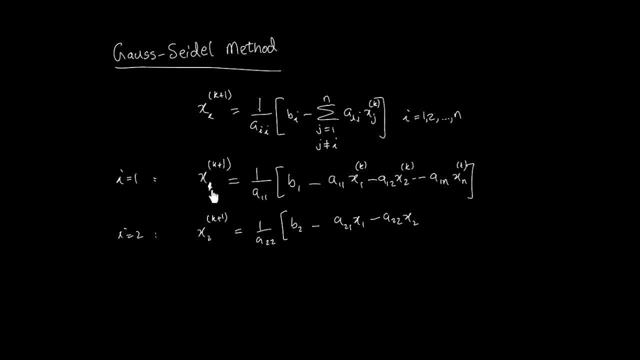 So now this is for i equals 1, so this gives us the iterative process for calculating the x1. For instance, k plus 1 is equal to all of this. fine, this is okay. but here is where it gets interesting. If you see this here: x1k, x2k, first one, no problem, we use the initial guess and we calculate x1k plus 1.. 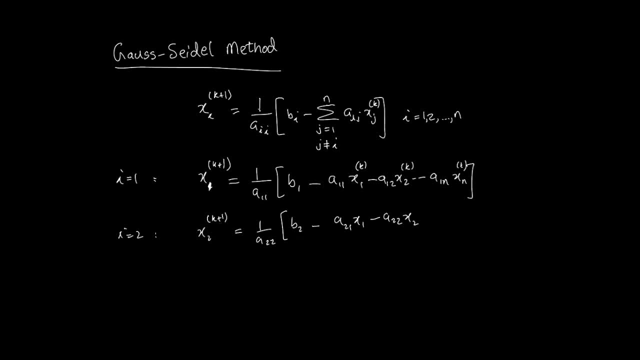 Now, if you notice here, when I go to x2k plus 1, b2, and there's x1 again. but wait a minute, why should I use x1k when I already have k plus 1?? You see what I mean. So if I were to say here k plus 1, I actually have already calculated it. so why not use the updated value of x1k plus 1?? 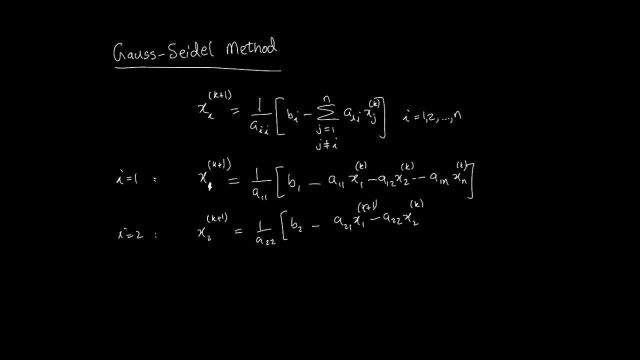 Now, of course, the remaining, all of these x2k minus dot, dot dot, minus a2n x2k. the remaining, I don't have them, so I'm just going to use this Now in the same way when I go to the next one. in fact, let me show you this: 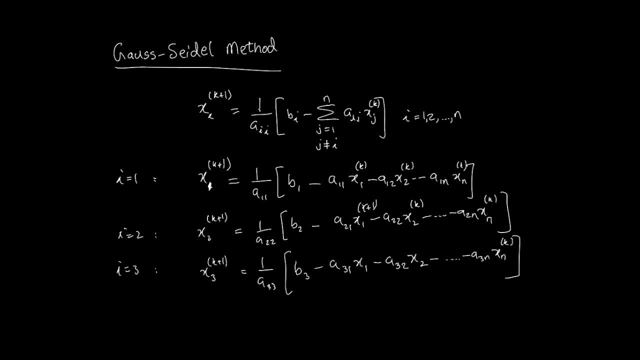 So here's the next one Now in x3, you see, I already have x1 and I have x2.. So rather than using k here, what I can do is I can say k plus 1 here, because I have it. 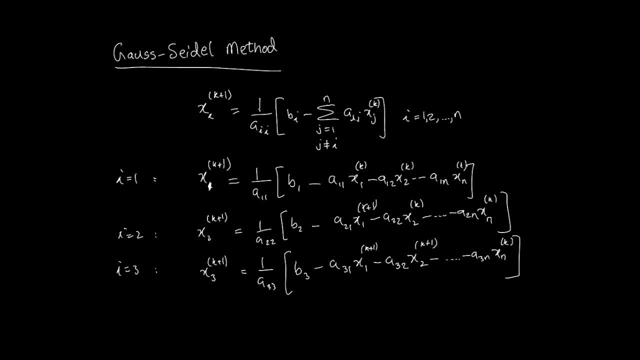 And same goes for x2, I can use k plus 1 because I've already calculated it, But x3 onwards up to xn, we'll use the k because we haven't updated, we don't have the values for x2.. 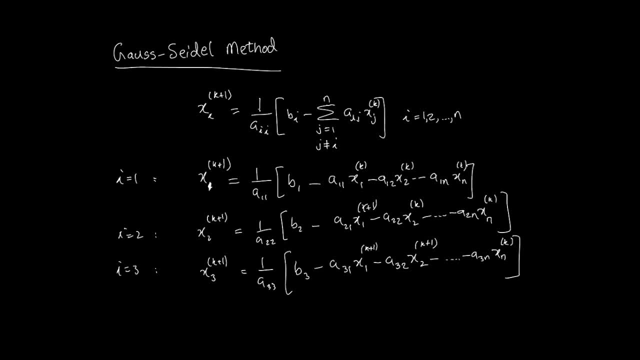 So what you can see is there is a. There is an interesting pattern developing here Is if we see, if we look at, for instance, this first one. So the pattern is that if you see here, when we're at x2, okay, the j's that are less than i, we can actually update them, because here this is 1, I can update it. 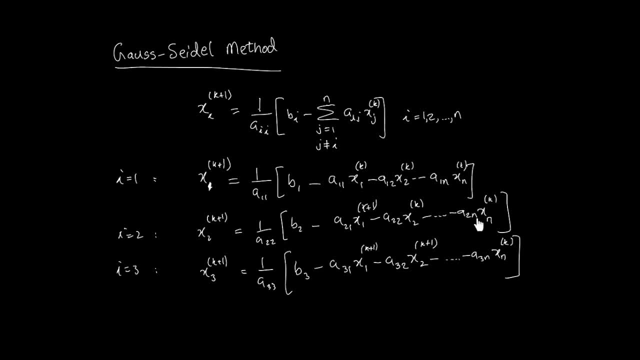 But once it becomes equal to this x2 and onwards, they're not updated. But, and similarly, when I go down here, if you see, this is 3.. So this 1. This 1 is less than 3, so this is a k plus 1 usable, and the 2 is also k plus 1 usable. the 3 that's equal to it is not. 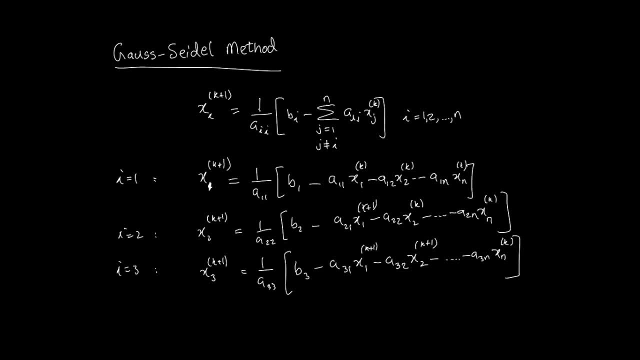 So what it seems to be saying is that I can actually set up two summations here: one for those- i sorry, j going from 1 to, in fact, i minus 1, okay, and the other one going from so or sorry onwards. 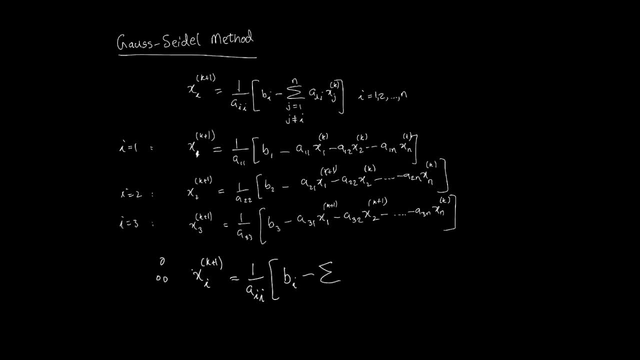 Let me show you what I mean. So what I'm trying to say is that I can do this: sum from j equals 1, right up to 1 less than the i, okay, In other words, whatever this is. so this is the i, so I can go up to i minus 1, no problem. and what I'm going to do there is this is aij, of course, but the xj that I have here. I would use the k plus 1th iterate, because I have already calculated them. 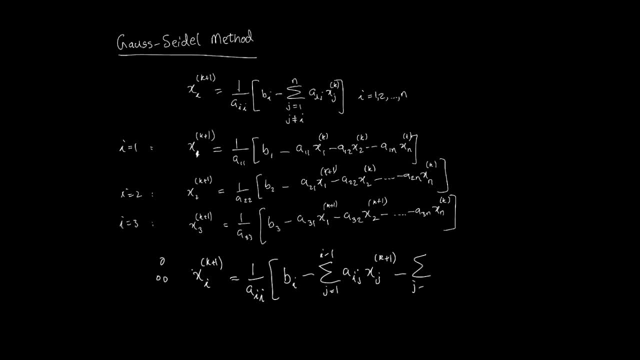 And then, of course, I'll have the, The remaining values, which will go from j equals- remember, I can't use i, i is already, i is over here. so that means that I'll continue with j equals, i plus 1, in fact all the way up to n- and then I have my aijs and xj, and that'll be just the kth iterate. 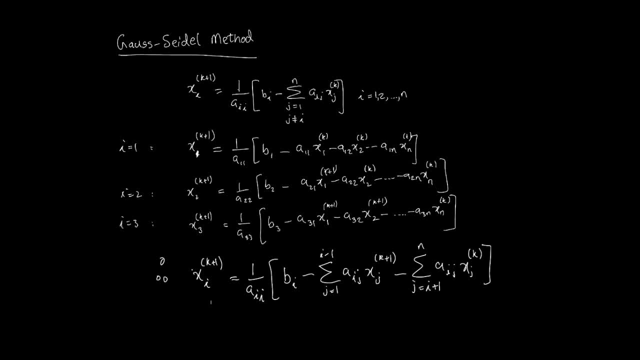 So this gives me a new iterative process, which actually is smart, because the point is: look, if I have the updated value, why shouldn't I use it? In fact, if I have the updated value, why shouldn't I use it? 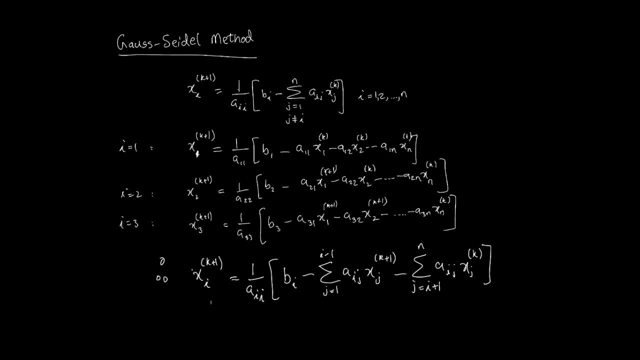 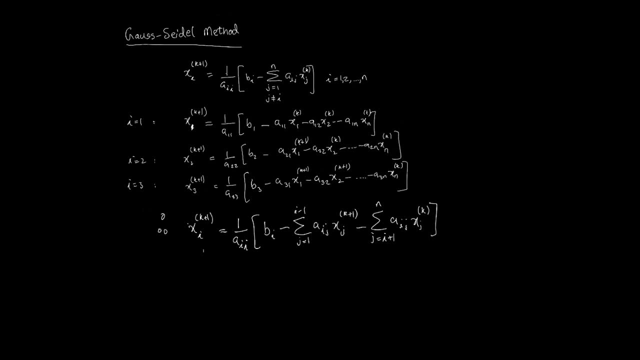 In fact, if I have the updated value, why shouldn't I use it? Because I would think that would actually speed up the iterative process and help converge faster. and that's in fact, what does happen in Gauss-Seidel. Gauss-Seidel is significantly faster than the Jacobi method. 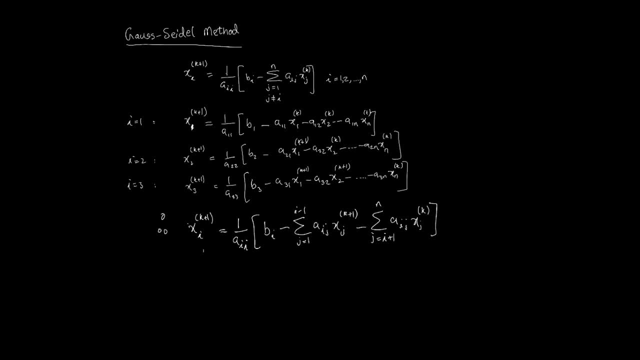 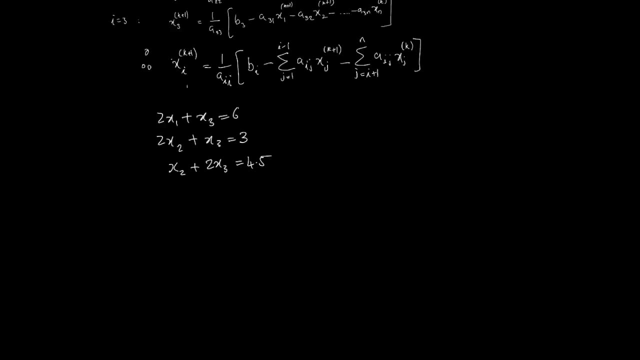 So let's try to see that in action, with the same example that we did for the Jacobi. so let's do that next. So here's the example again. Now, this is the same example, but we're going to solve this using the Jacobi method. 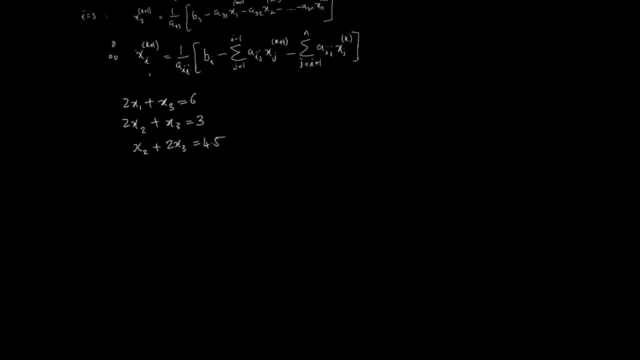 So the iterations will work something like this: From the first equation we have nothing yet, so we'll just write that as k plus 1, and that's our x1,. x plus 1, and that's equal to 6 minus x3, which is the kth iterate divided by 2, of course. 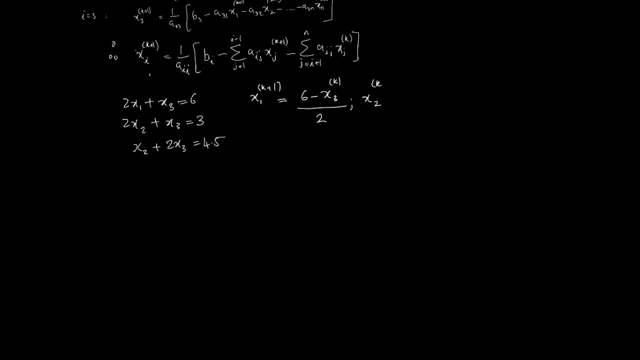 The next iterative process is for x2, k plus 1 is equal to, and this one also basically is just 3 minus x3.. Now, since we haven't calculated x3 yet, there is no, We'll just use k here. and that also is divided by 2.. 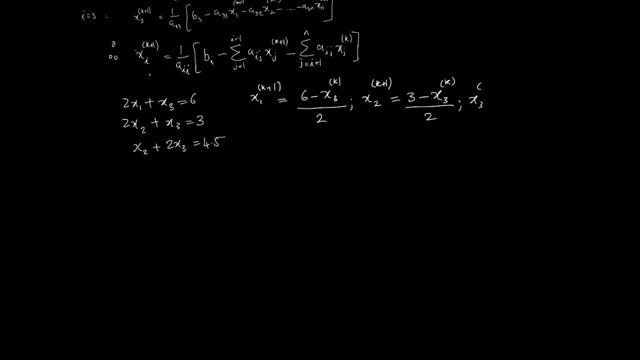 So there's no difference so far. Now the interesting thing happens when we get to x3.. If you notice, in x3, it's 4.5 minus x2.. Now x2 is already calculated here. So therefore we can easily say x2, k plus 1 on here, and that's divided by 2.. 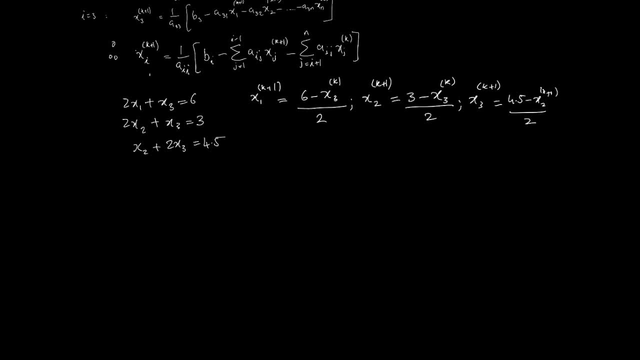 So the minor difference between this and the Jacobi would be that, Jacobi, this one, this is just x2, k instead of k plus 1. And that does make a lot of difference. But let's look at how we would proceed to calculate this. 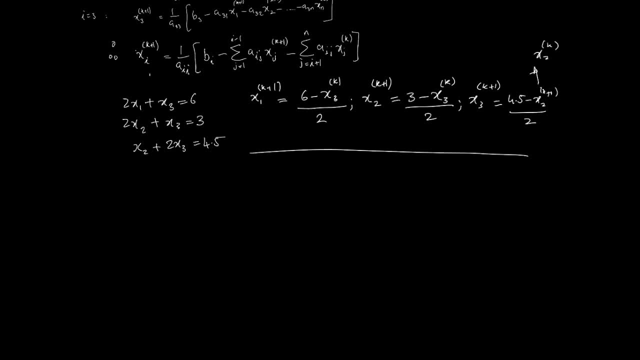 So in this case, if we were to tabulate this for instance- and here would be our k, So we'll go with again the same initial guess, vector 0, 0, 0. So for k, 0.5 minus 1.5 is 3 divided by 2.. 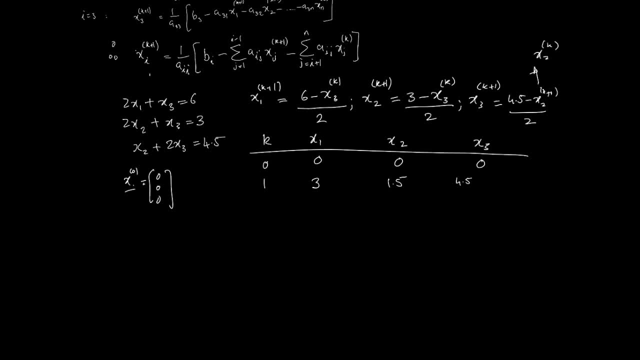 Gives me. So I'll just show you here what I'm saying: 4.5 minus 1.5 divided by 2, and that gives me actually 1.5.. So you'll see, here is the change begins to happen, the difference. 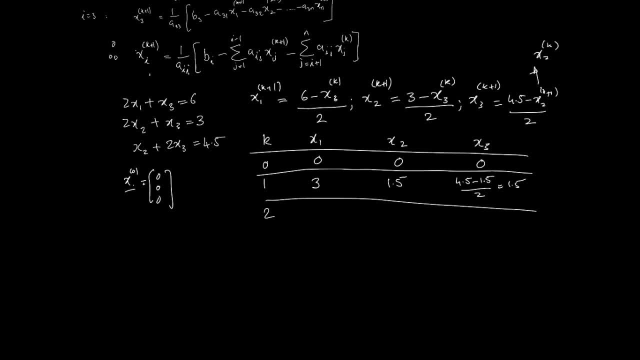 So if I go further now here, the next iterate, the second iterate is going to be Already. I'm going to see a difference now, because I'm going to say 6 minus Now, of course, x3, and x3 is 1.5, so I'm going to get 2.25 in this. 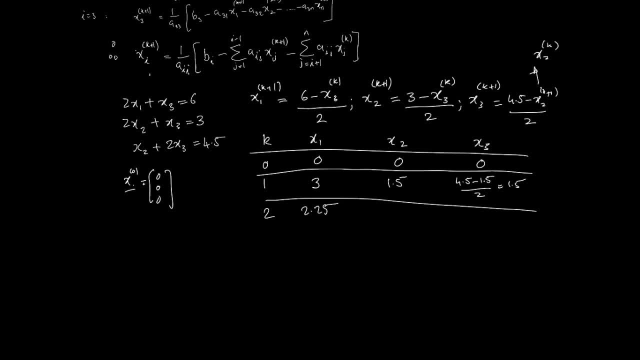 So it's 2.25, and over here, when I come here, of course, it's still. It's 3 minus 1.5, so 1.5 divided by 2 is 0.75.. So that becomes 0.75.. 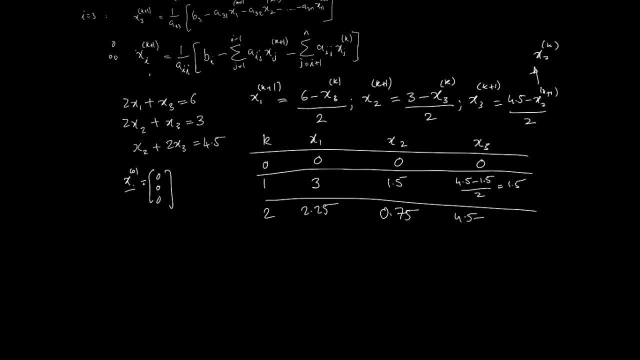 Now, here again. I'll show it to you Again: 4.5 minus. Of course. we're going to use this, as we did use this one here. So I'm going to use this over here. so I'm going to get 0.75 subtracting from this. 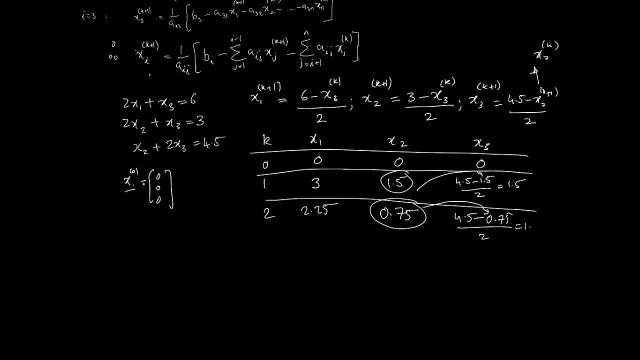 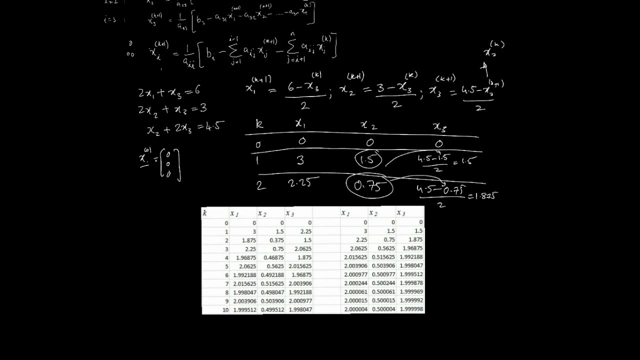 divided, Divided by 2, and that gives me 1.875.. So in this way I can proceed and I'll show you 10 iterations of this next, alongside with the Jacobi, to show you the difference. So here in the Jacobi on the left that you see over here, this is the Jacobi and you. 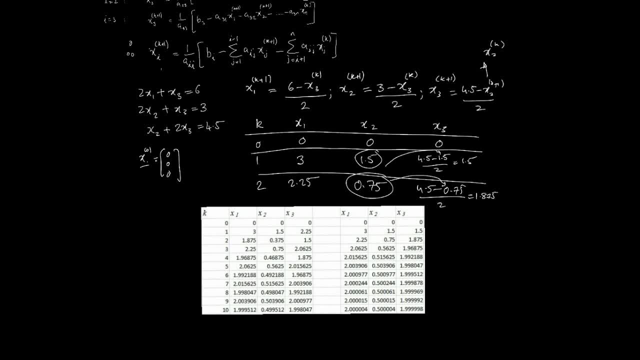 can see that it's just at the 10th iteration, getting quite close to the actual answer, which is 2.52.. 2.- 2.. On the other hand, in the Gauss-Seidel you can see that happening almost. here is where you'd say this: 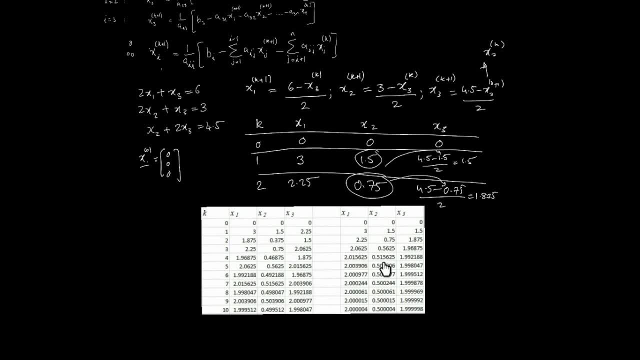 Actually, even this one is very close. So, third and fourth iterations, we're very close to the actual answer, and then after that it becomes even closer, of course. So it's a much faster method, almost going at. So what you'd really like to do is to compare.